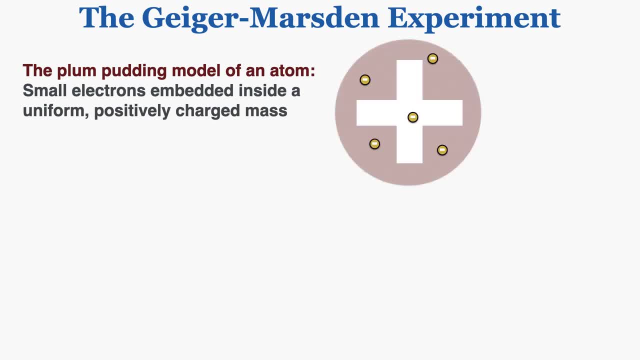 but the plum-pudding model of an atom said that an atom was small electrons embedded inside of a uniform positively charged mass, something like this picture right here, where you have electrons stuck in a spherical low-density nucleus. This is a picture of a plum-pudding model of an atom. 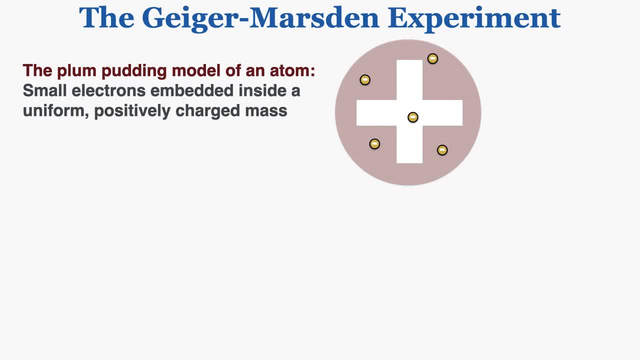 positively charged mass. The reason it's called the plum-pudding model is that this physically looks like a plum-pudding, with little pieces of fruit embedded in the cake, And the Geiger-Marsden experiment allowed us to move from this model to a more correct model of an atom called the. 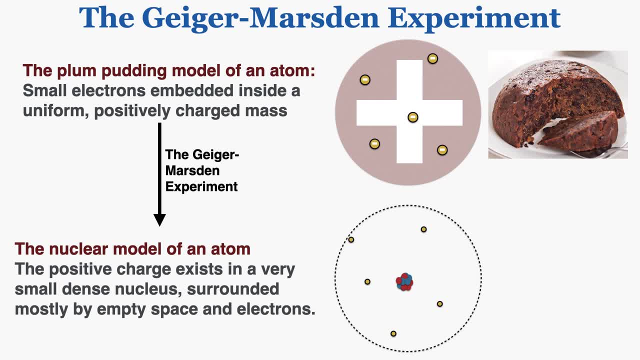 nuclear model, where the positive charge of an atom exists in a very small, dense nucleus surrounded mostly by empty space and electrons. So the experiment showed that the plum-pudding model was probably not correct and hinted at the nuclear model instead. In the experiment itself, 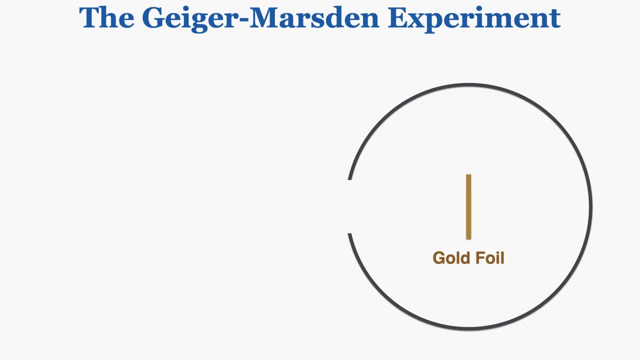 scientists took a very thin film of gold foil and placed it inside of a circular screen. This is an overhead view of the experiment. I want you to imagine that when you're looking at this, you're looking physically down at a table that you're standing over and the circular gray screen is. 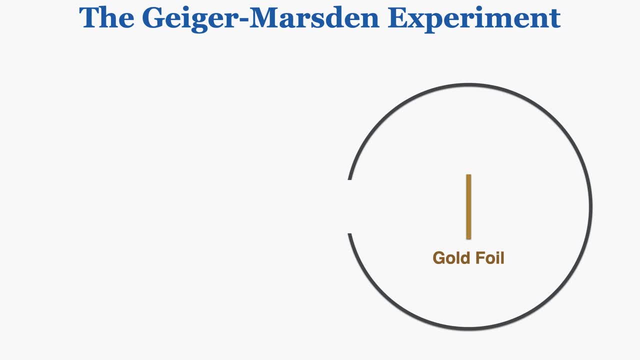 resting on the table horizontally and the gold foil is placed in the middle. The reason why the scientists used gold specifically is that gold can hold its structure while still being incredibly thin. The scientists doing the experiment were pretty confident that the gold foil itself was. 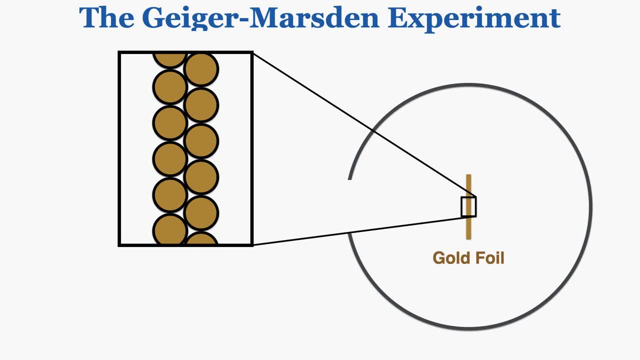 actually probably only two or three lines of atoms thick. So any interference with these atoms would be the result of interference with just a single atom, or maybe two atoms at the most. So they knew that whatever happened in the experiment would be the result of interference with just a single atom. 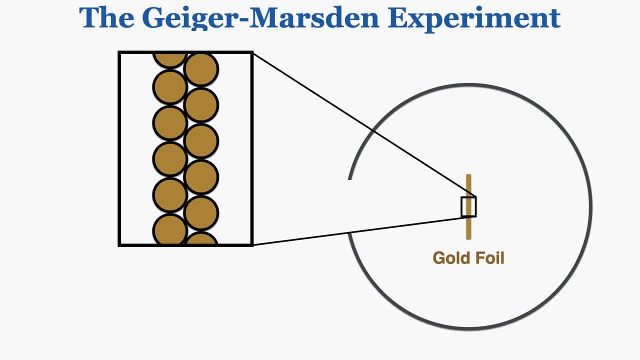 rather than the result of the interference of very large amounts of atoms, because there could be other factors there affecting the experiment that we didn't know about. but if they only dealt with individual atoms they could get a pretty clear idea of the shape of the atom Scientists 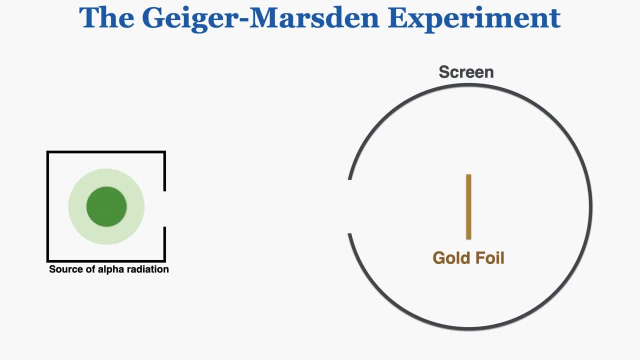 set up a source of alpha radii as a form of radioactivity, which they called radioactivity. This just a radioactive substance inside of a lead box, and they created a very small opening in the box and the substance would emit alpha particles in every direction, but the only alpha particles that 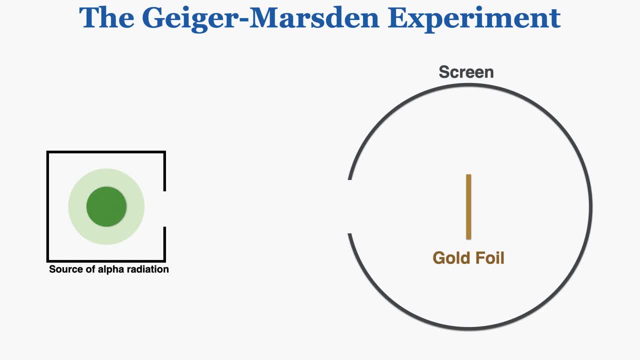 could actually escape the box would have to be going straight through that hole. so they would continue along their same path and eventually go straight at the gold foil. Without the gold foil there, they knew that what would happen is an alpha particle would be emitted, hit the screen and they. 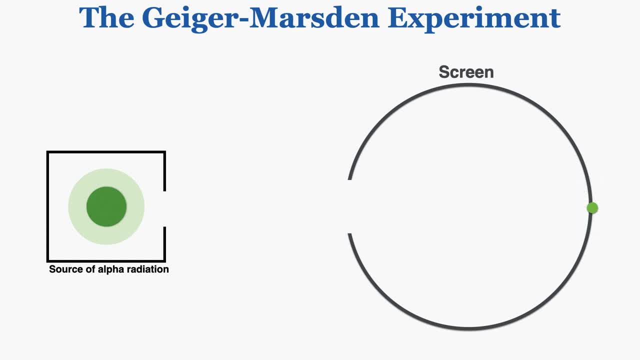 would be able to see on the screen exactly where the alpha particle impacted the screen. There would be a little mark on the screen that appeared, so I'll use a green dot to represent what those marks look like. We now know that alpha particles are two protons and two neutrons, so they're 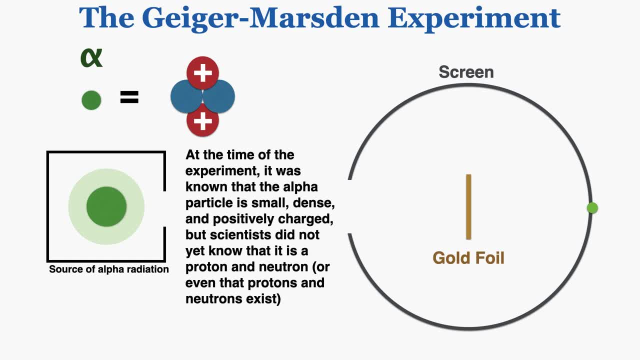 positively charged. At the time of the experiment it was known that the alpha particle is small, dense and positively charged, but scientists did not yet know that it's a proton and a neutron, because they didn't even know that protons and neutrons existed at the time. So they were trying. 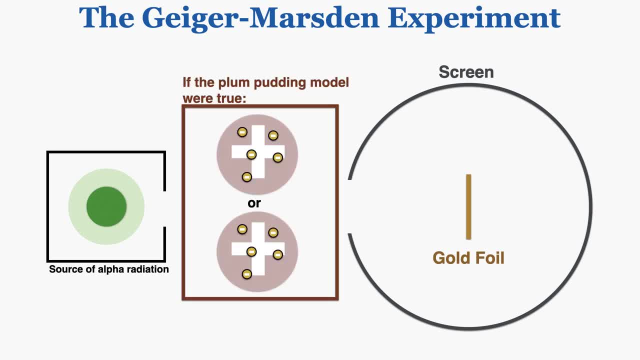 to confirm the plum pudding model of the atom. and if the plum pudding model were true, one of two things would happen. One possibility is that all the alpha particles would move through the atom. Because scientists assumed that the atom was very low density. the alpha particles could probably just effortlessly. 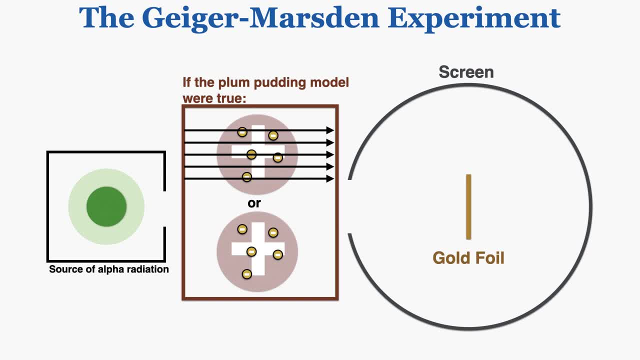 move through to the other side, because they were much smaller and denser. The important thing here, though, is that the plum pudding model predicted that the atom was uniform. There's no small dense nucleus in the center, surrounded by empty space. Instead, the entire atom is just the same low. 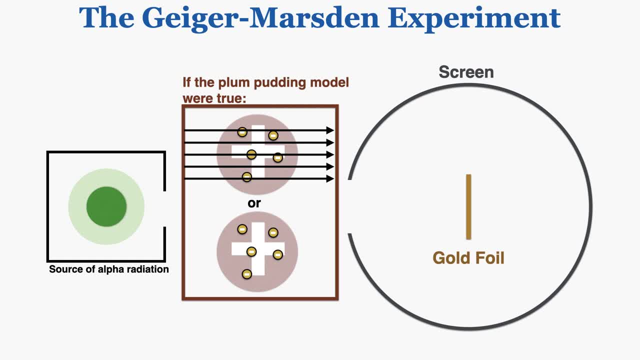 density object, And so no matter what part of the atom was in the center of the atom, it was not square or whoever the smaller the particle is at our center. this is a constant. So all the elements in the center and the upper part of the atom are going to be the same, regardless of what. 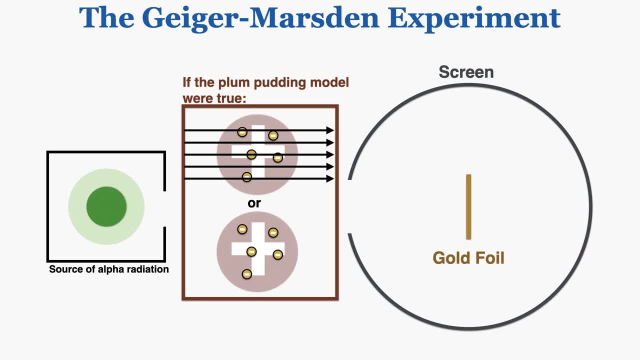 the specific part of the atom is going to be, And if the atom is moving or moving through a particle, that's the same. the top, middle and bottom paths that the alpha particles took should all be the same, going through the atom, regardless of which specific part of the atom they traveled. 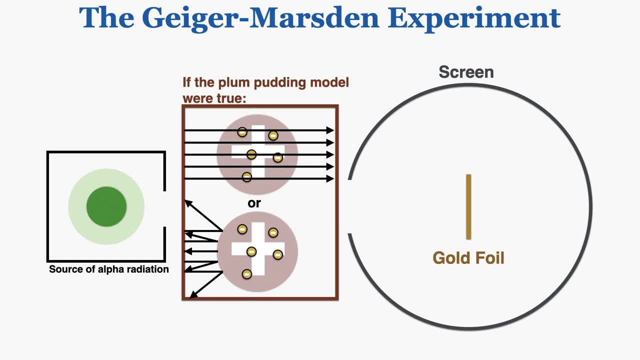 through. The other possibility was that maybe the atom was actually denser than alpha particles or dense enough for them to be repelled, So maybe all the alpha particles would be repelled back this way. This wasn't a serious assumption, but it was obviously a possibility in the plum pudding model. 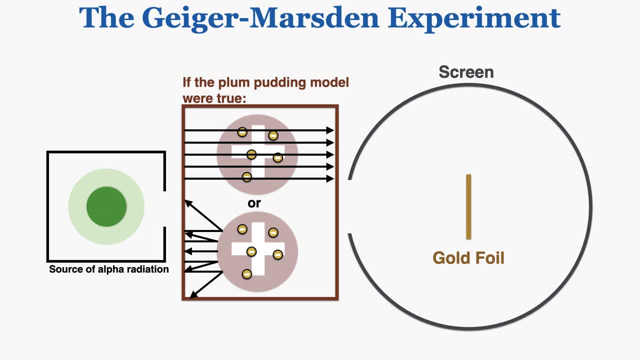 shouldn't matter. Same density everywhere, so it should always bounce off or it should always go through. So if the plum pudding model were true, we would expect one of these behaviors or the other. And it was known that the alpha particles were small and dense and that the atoms were 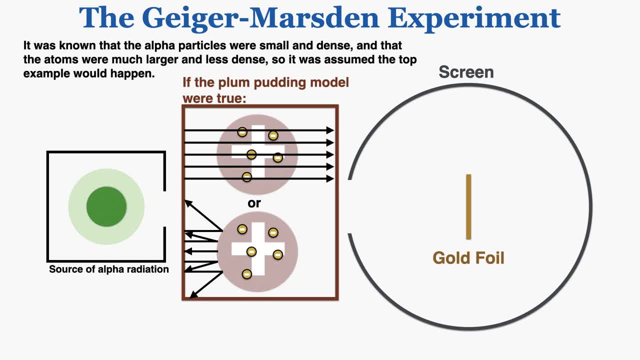 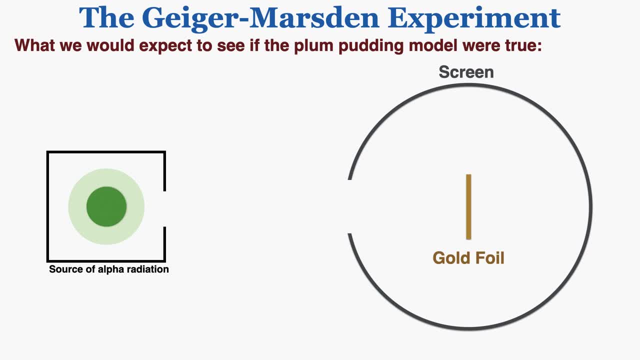 much larger and less dense, so it was assumed that the top example would happen. So, based on those assumptions, this is what we would expect to see if the plum pudding model were true. If we shot a lot of alpha particles at the gold foil, we would expect their imprints on the screen. 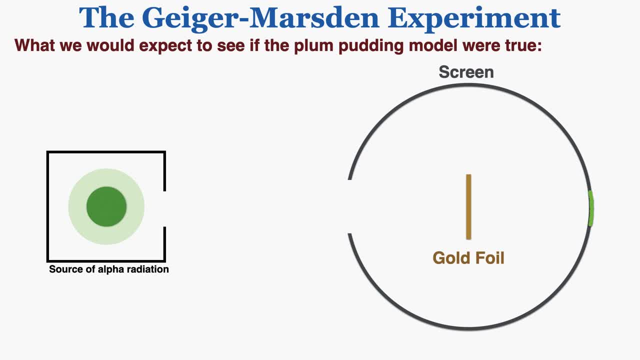 to appear here. The reason why we would expect them to see them here is that if all the alpha particles were able to effortlessly move through the atom, we would expect that all the alpha particles would follow this path through the gold foil, because the gold foil is just made of. 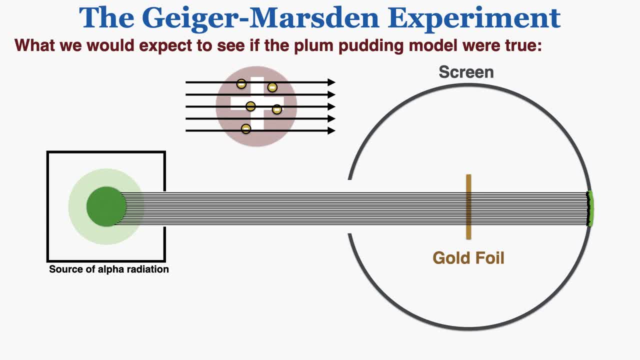 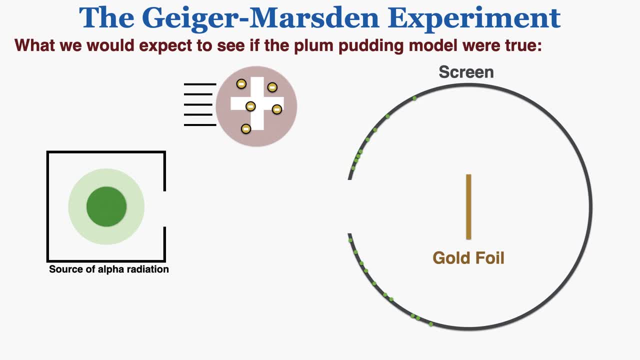 individual atoms, So we would expect them to appear there, on the other side of the foil. The other possibility- if the atom were more dense- is that this pattern would appear, because if the atom were more dense, all of the alpha particles would be rebounded off of the 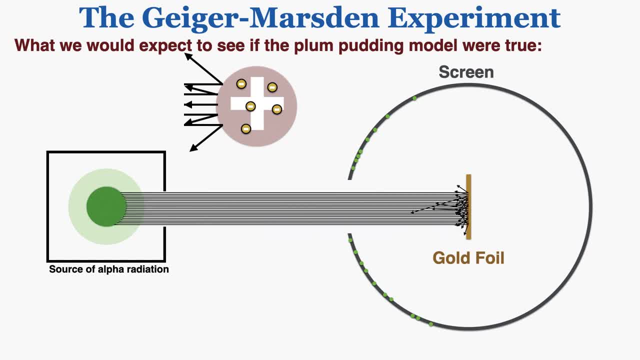 atoms in random directions, and so the alpha particles would be able to move through the atom like this. So we would expect one or the other pattern if the plum pudding model were true, but that's not what actually happened. Instead, we got this pattern here. You can see that most. 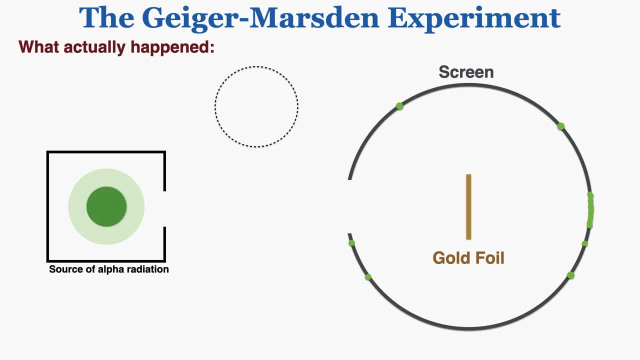 of the alpha particles did hit the other side, but there are a few that are off in strange directions and a few that actually bounce off the gold foil and exist on the left side of the gold foil. This hints at a pattern of the alpha particles moving through the atom like this. 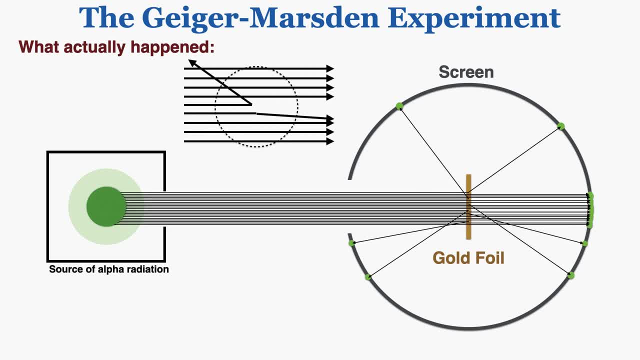 because when they came out of the source of the radiation, most of them moved straight through the gold foil, but a few bounced off in random directions and a few were even bounced backwards in the opposite direction, like that. So a majority moved through, but you had a few that bounced off in other directions. So if you look up at my 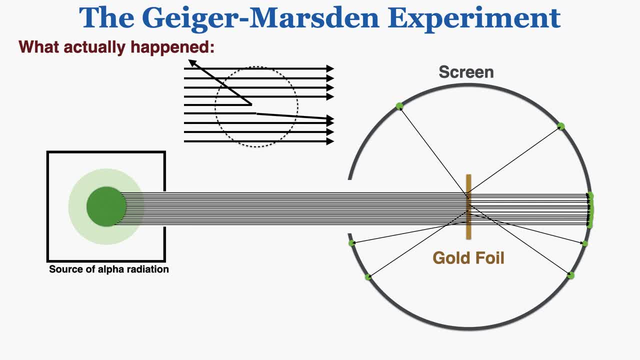 diagram of the atom. what this implies is that most of the atom is very easy for particles to move through, but there must be some very small, very dense spot where alpha particles are bounced off. that deflects alpha particles and pushes them away, and it's dense enough to be able to move. 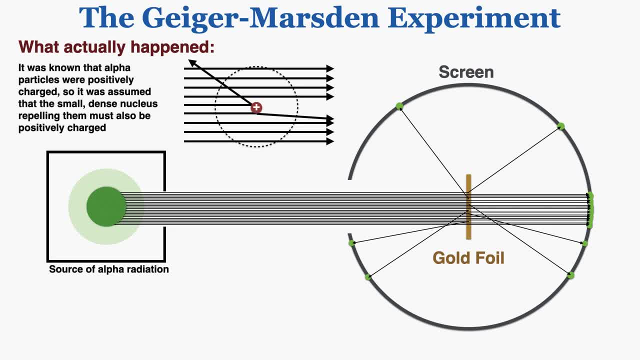 through. It was known that alpha particles were positively charged, so it was assumed that the small, dense nucleus repelling them must also be positively charged. So this pattern hinted that the plum pudding model was wrong and instead a nuclear model of the atom was correct Where most 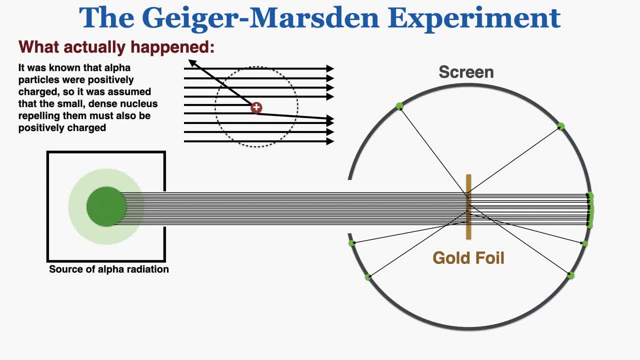 of the atom was empty space. that was very easy for alpha particles to move through. but a very small portion of the atom must be a small, dense, positively charged region that repels alpha particles. So this is how we got from the plumped nucleus to the positive nucleus, And so we got. 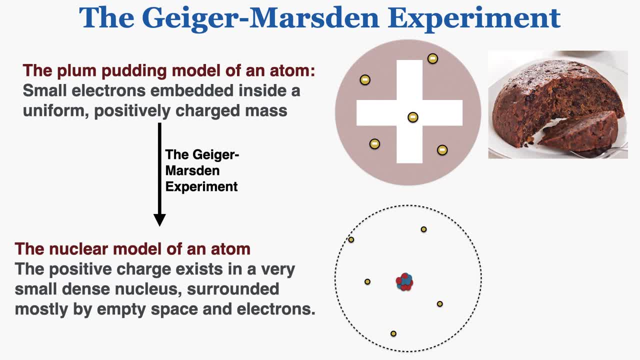 a very small, dense nucleus repelling them. but a very small portion of the atom must be a small plum pudding model of the atom to the nuclear model of an atom, And that's how the Geiger-Marsden experiment helped us progress from one to the other.